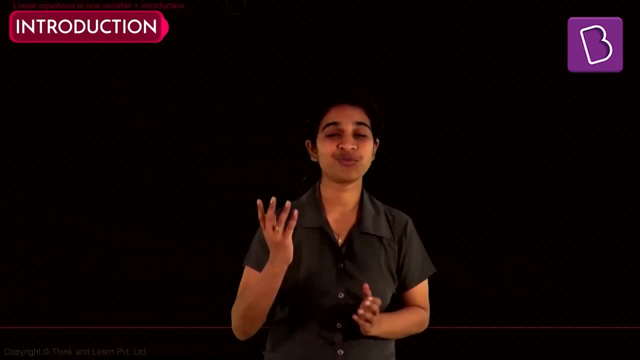 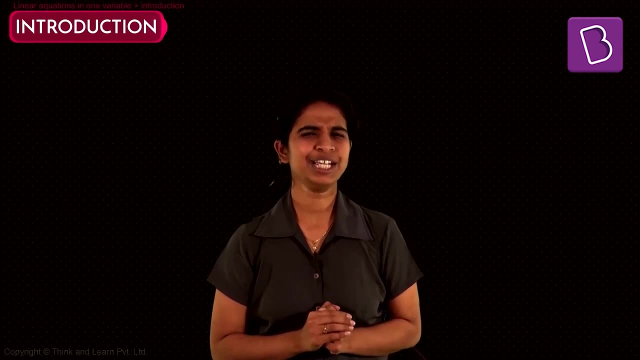 That is what an equation tells you. Now an equation could be about fun things like my height and such and scored. Or it could be about more boring things like algebraic expressions. Do you remember 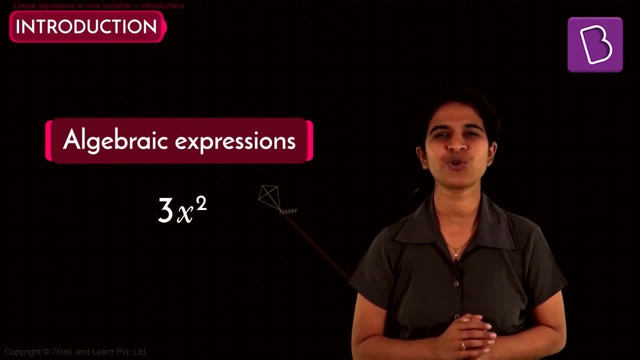 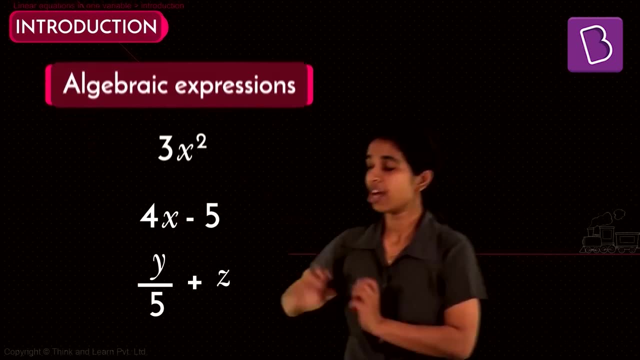 algebraic expressions you saw things like 3x square 4x minus 5 y by 5 plus z and so on these were all algebraic expressions now you pick any two of these and put an equal to sign in between 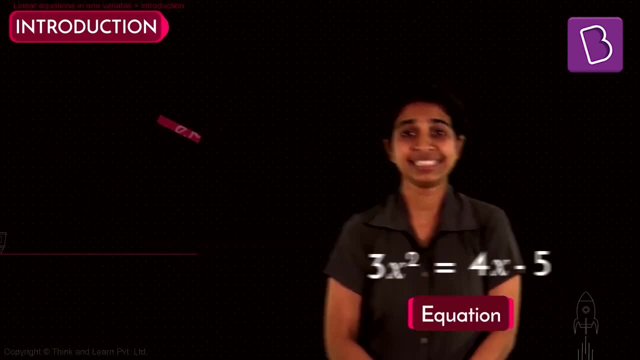 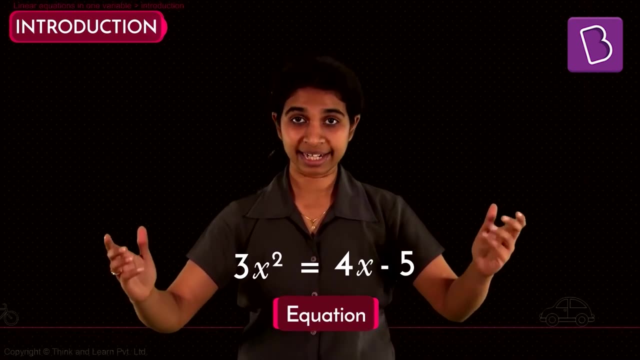 and voila you have an equation that's what an equation is it says the two sides of the equal to sign are exactly the same it doesn't tell you what is on the two sides it could be sentences it could be algebraic expressions it could be numbers it could be anything that's what an equation is 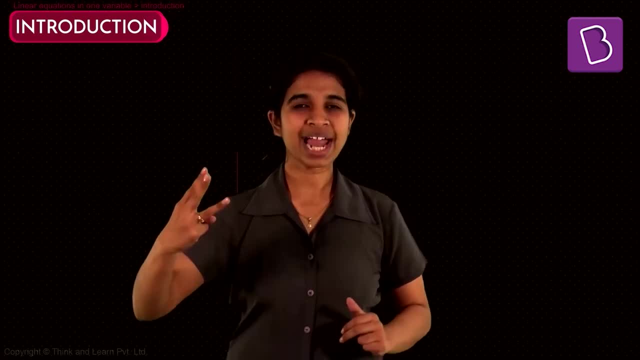 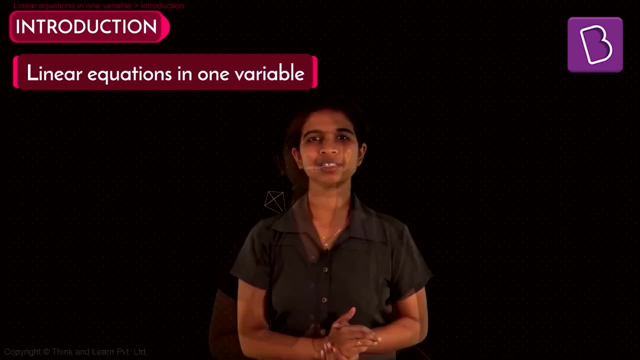 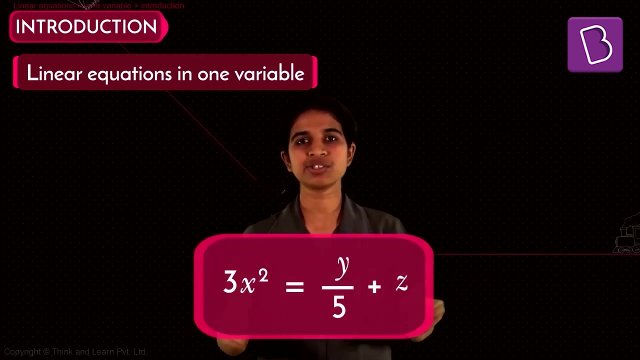 so we have an equation we've understood what an equation we had three words to understand right linear equations in one variable now variable you already know what variables are a variable is nothing but an unknown a quantity which is not known so all the x y's and z's that 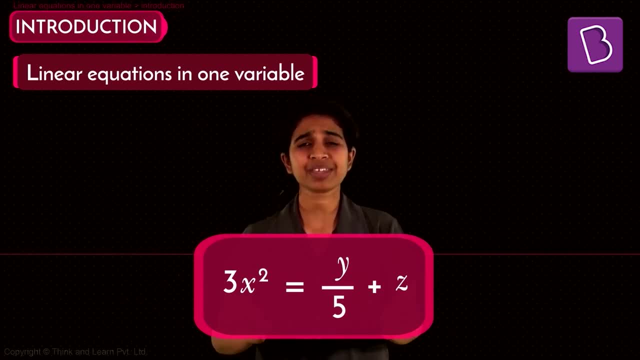 you see in this expression are nothing but variables any unknown quantity that is a variable we are going to deal 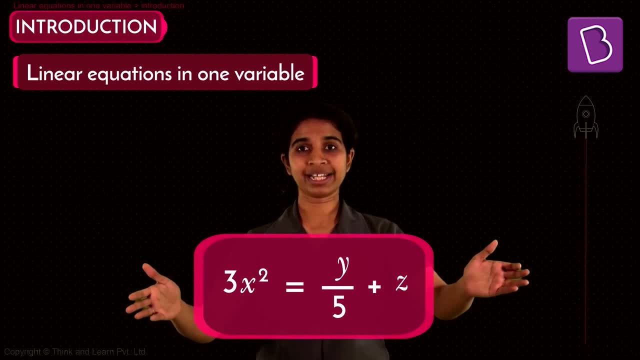 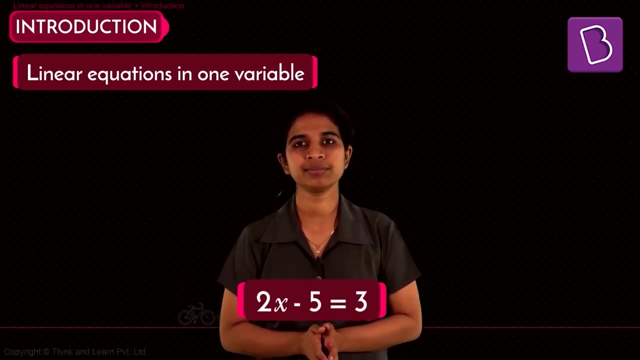 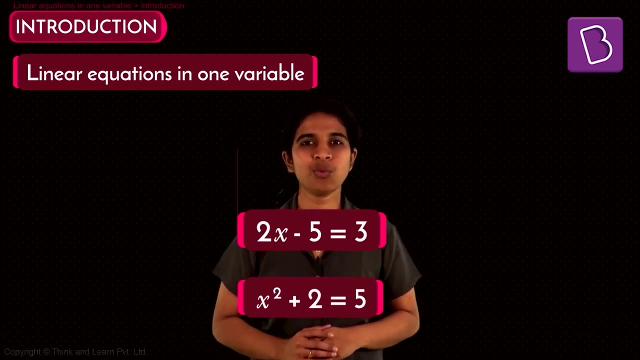 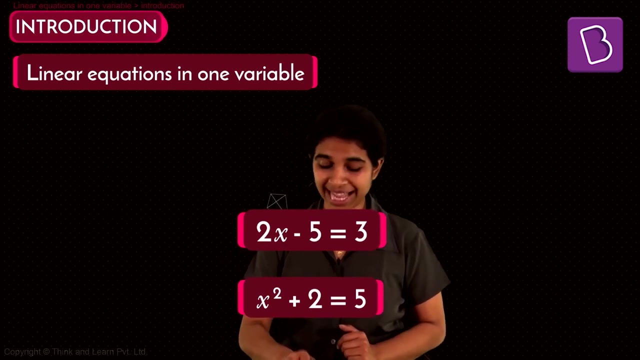 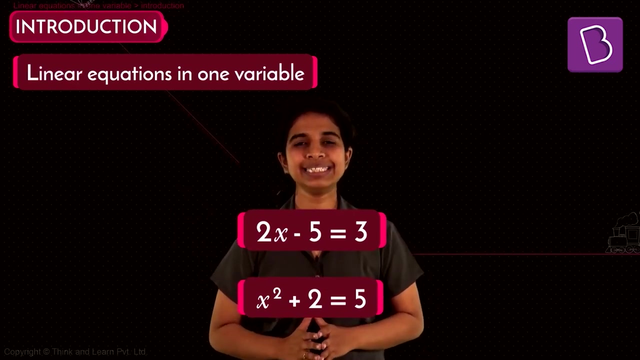 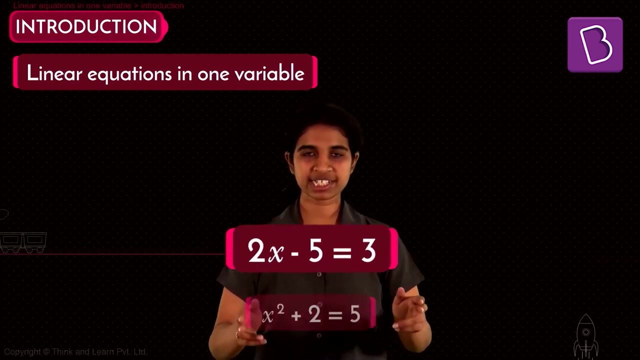 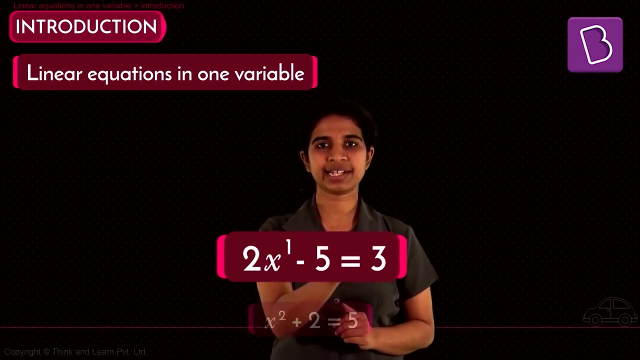 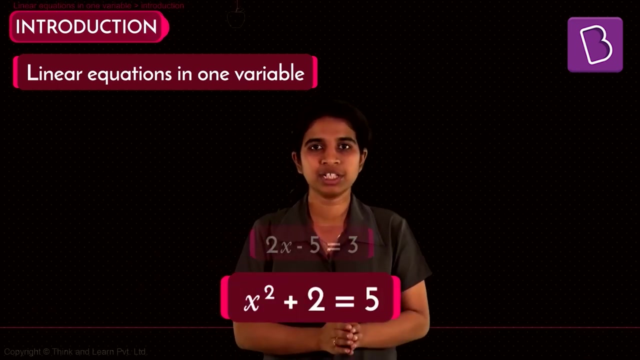 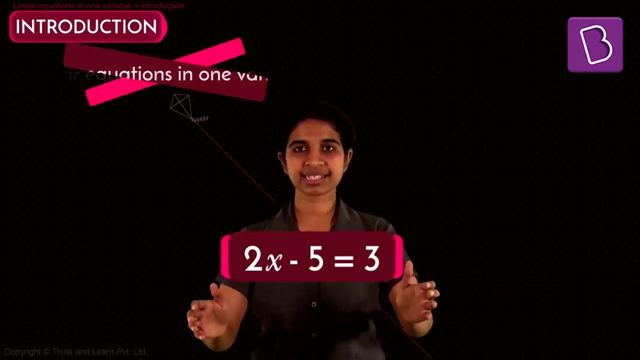 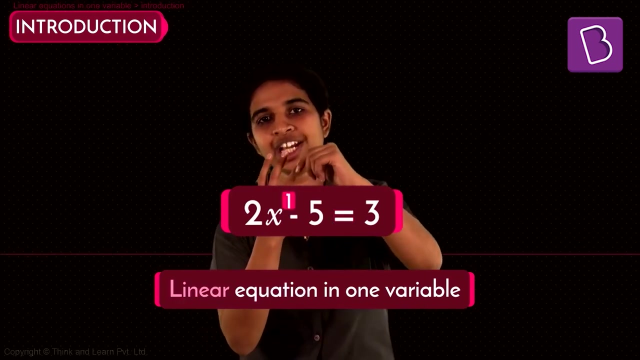 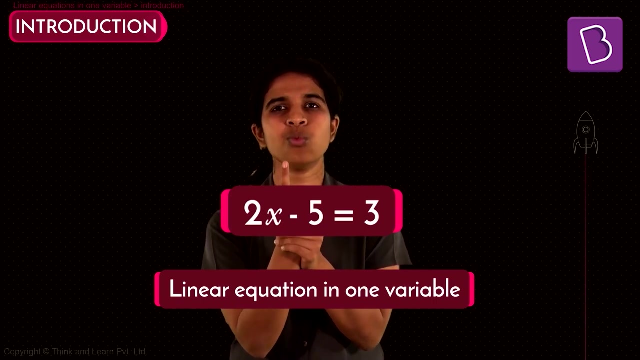 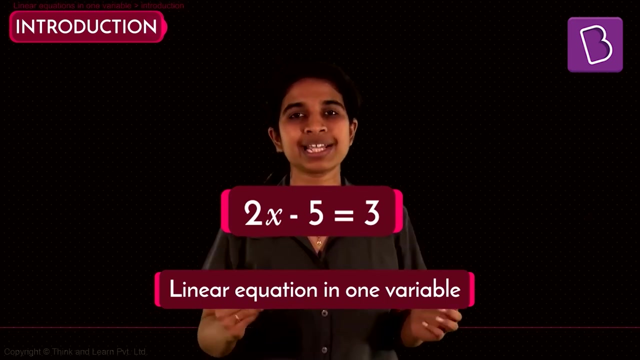 with equations in only one variable so we don't want an equation like this with three variables we want a simpler one with just one variable let's say 2x minus 5 equal to 3 it's an equation in one variable x square plus 2 equal to 5 again an equation in one variable so there's only one unknown quantity everything else is known all the other things are known great so it has an equal to sign it is an equation it has only one variable so it is in one way now what is this linear what does linear tell you linear is nothing but if you look at the highest power of the variable in the first case look at the first equation what is the highest power of x 1 right because only x is nothing but x raised to 1. so the highest power of x here is 1. in the second expression you have an x square here so what is the power of x x is raised to 2 or the power of x is 2. so this the second expression here the second equation here is not a linear equation because the power of x is 2. so get rid of this this is a linear equation in one variable satisfies all three of our conditions is an equation it's linear has only one variable so that's what a linear equation is it has the highest power of the variable is 1 and why do we call this as linear is something you'll learn later all of these expressions are linear and they are not linear if you start visualizing them they'll be straight lines which is why we call them linear like a line